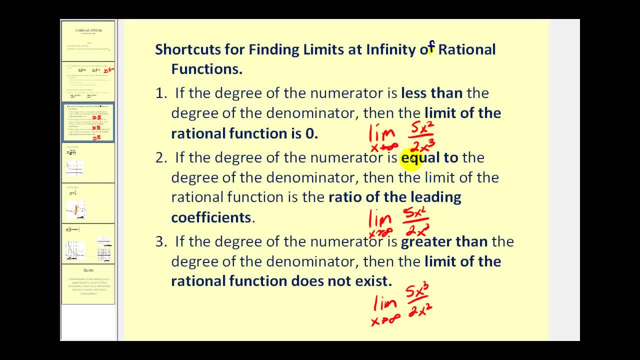 if the degree of the denominator is larger than the degree of the numerator, the denominator is growing faster and therefore this will equal zero. The second case is when we have the degree of the numerator is equal to the degree of the denominator, and if this? 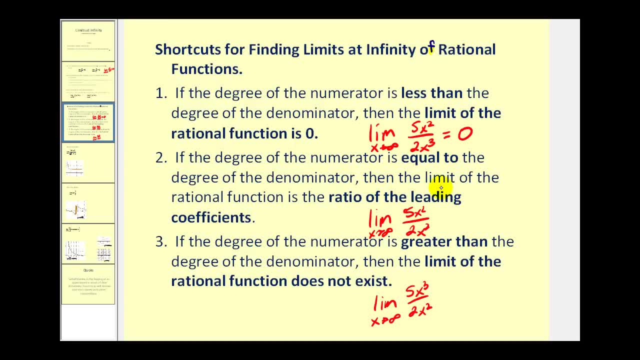 is the case, then the limit is equal to the ratio of the leading coefficients. So here's an example where they're both degree two, fluorescentappscom two, and the ratio of the leading coefficients is five to two. therefore this limit is equal to five halves. And then, lastly, if the degree of the numerator is greater than the degree, 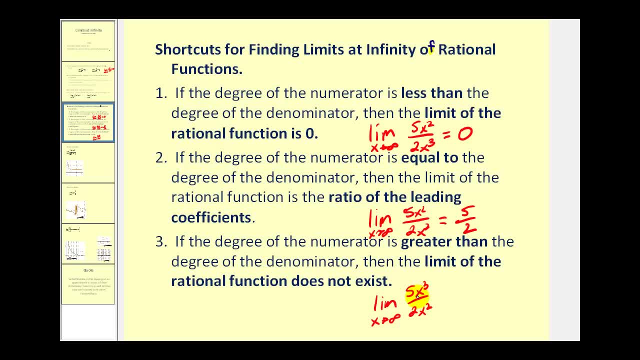 of the denominator, then the limit does not exist. So if this has a higher power, this is growing faster than the denominator and therefore would approach, in this case, positive infinity, which does not exist. Okay, let's take a look at three additional examples. 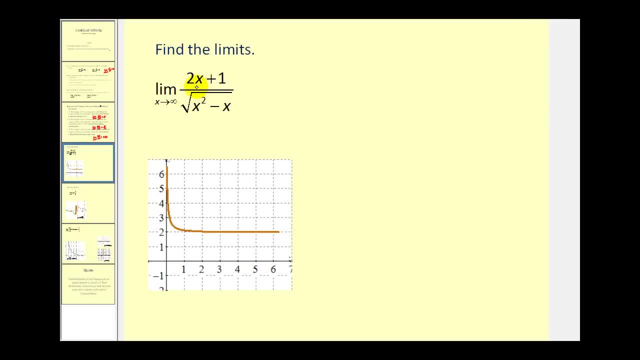 We have the limit, as x approaches infinity, of the quantity two x plus one divided by the square root of x squared minus x. Let's take a look at the graph first. It's pretty easy to see from the graph that as x approaches positive infinity, this function approaches. 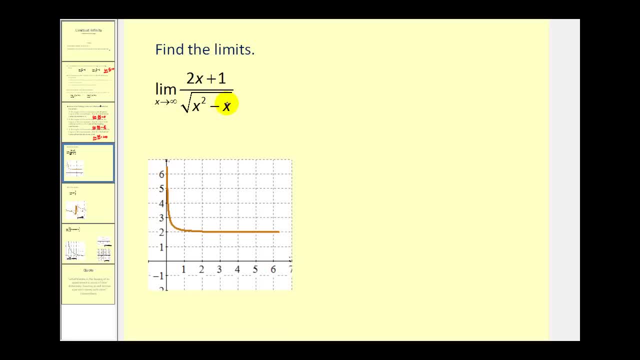 the value of y equals two, and that is what this limit is equal to. Let's take a look at a couple other ways to determine this limit. The most general way is to divide by the highest power of x in the denominator. Well, we have an x squared in the denominator, so we'll divide everything in the denominator. 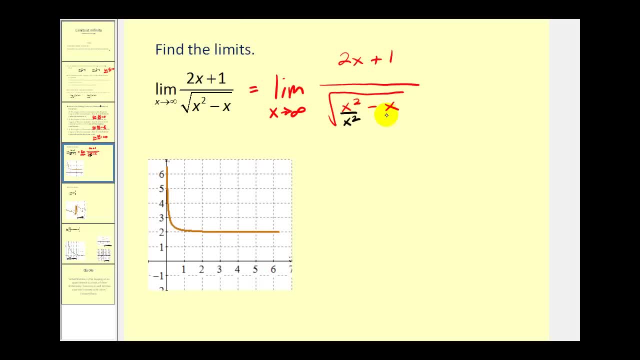 by x squared. But remember this: x squared is underneath the square root. The square root of x squared is equal to x, so when we go to the numerator we'll have to divide by x Again. the reason this looks different is because the square root of x squared is 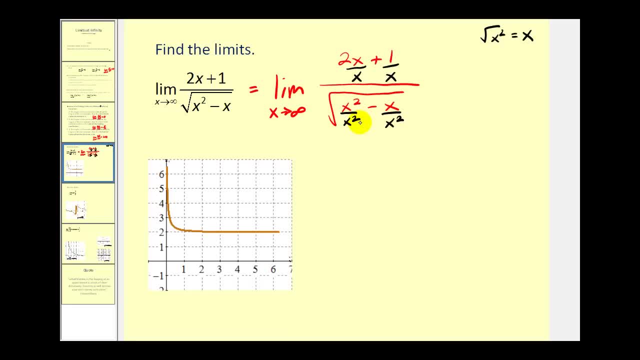 equal to x. So we are dividing both the numerator and denominator by the same value. Let's go ahead and simplify this. We would have two plus one over x. I'll divide it by the square root of one minus. this would be one over x. Well, this approach is zero. This approach is zero, So we're left with. 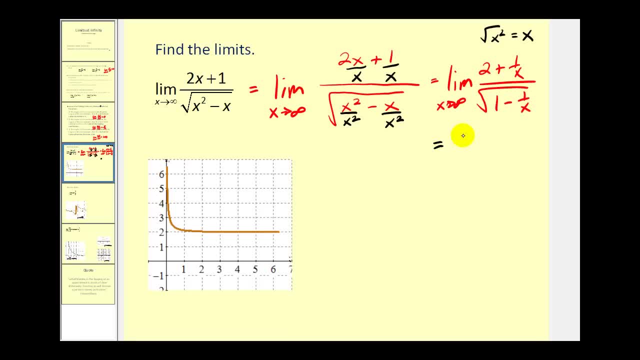 two over the square root of one, which of course is equal to two. And a third way to evaluate this limit. using this shortcut, you can think of this as having degree one, because the square root of x squared and this also has degree one, So the ratio of the leading. 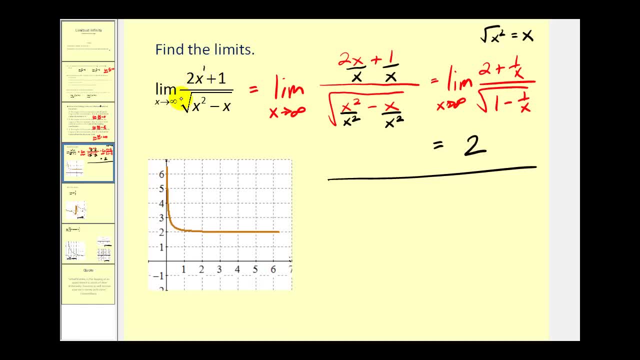 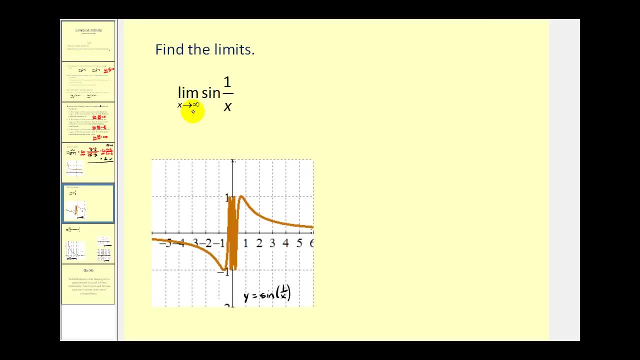 coefficients would be two divided by the square root of one, which of course is also equal to two. Let's go ahead and take a look at another one. Here we have the limit, as x approaches infinity, of sine: one over x. Well, by now we should know that one over x is going to 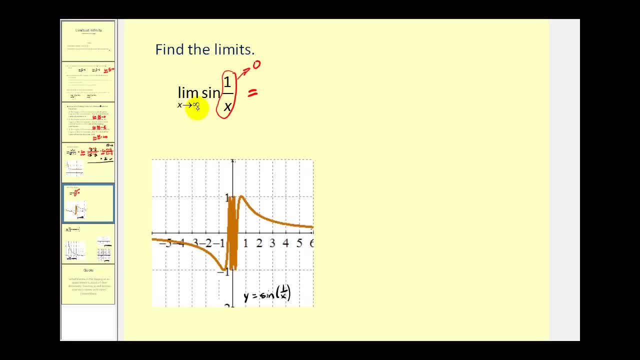 approach zero. as x approaches infinity, We have one over an increasing denominator. Well, this would equal the sine of zero, which is equal to zero, Or graphically you can see, as you approach positive infinity, this graph is approaching. y equals zero, or the x-axis. 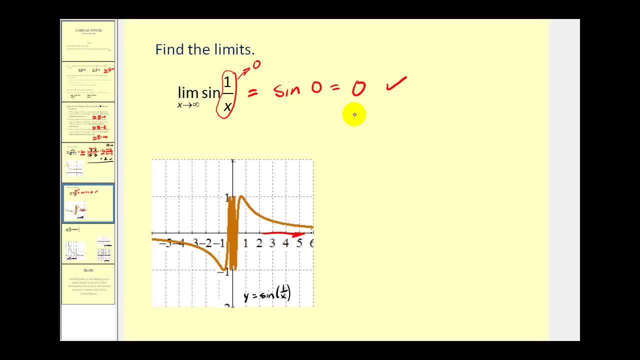 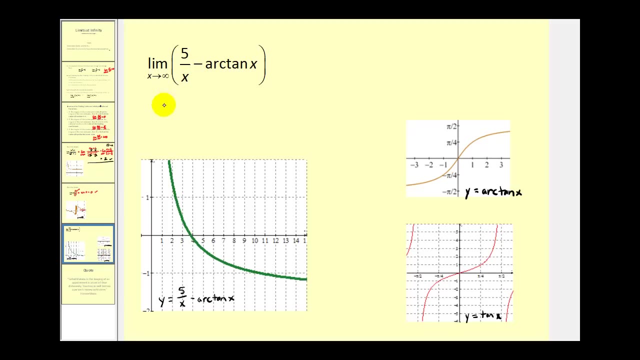 therefore, this does verify our limit. We should also notice that this graph does have a horizontal asymptote of y equals zero, which is the same as the value of this limit at infinity. Okay, let's take a look at one more. Here we have the limit, as x approaches infinity, of five divided by x minus arctangent x. So 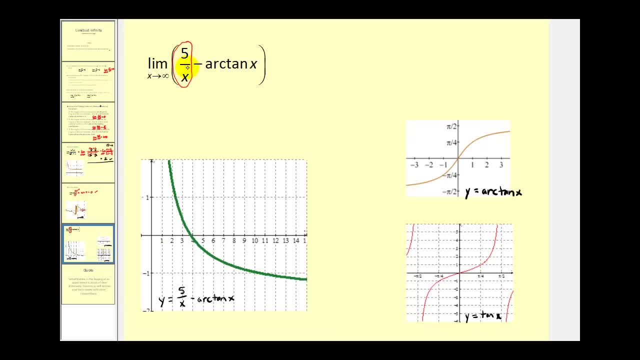 we should realize now that five divided by x, as x approaches infinity, is going to approach zero. So the real question becomes: what is negative arctangent x going to approach as x approaches positive infinity? And again, there's a couple ways to analyze this. If 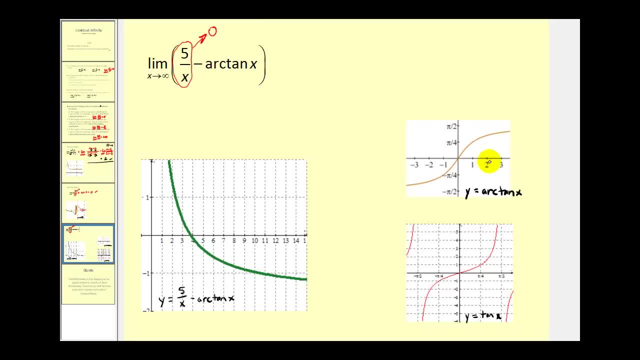 we were to graph arctangent x as we see here. it's pretty easy to see that as x approaches positive infinity, the function value is approaching pi divided by two. So this would equal zero minus pi divided by two, which is equal to negative pi over two. Remember that this x value here is the tangent function. 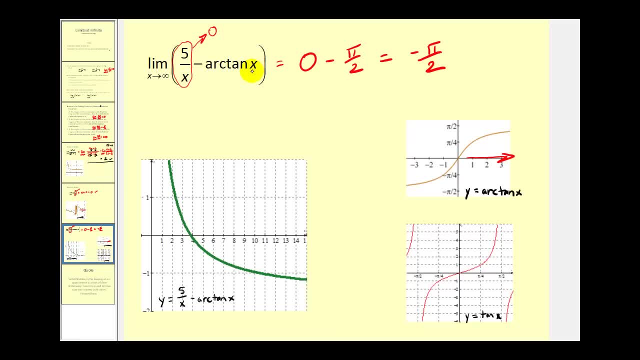 value and arctangent returns an angle. So another way to think of the same thing would be to look at the graph of the tangent function. As we see, as the tangent function value approaches positive infinity, the angle is approaching pi over two. So there are several ways to analyze this limit and I think if looking